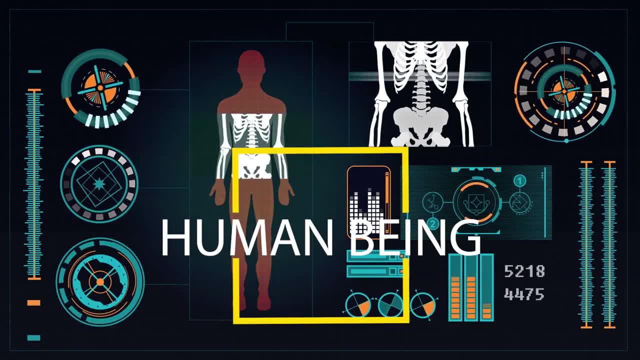 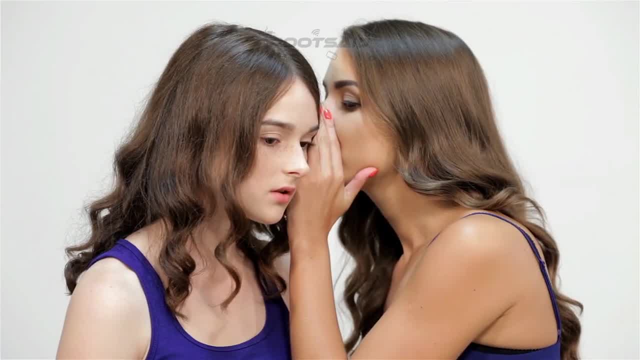 robotics. Imagine: a robot is like any other organism, Like a human being. We have sense organs. We see things with our eyes, we hear things with our ears, feel with our skin, taste with our tongue and smell with our nose. 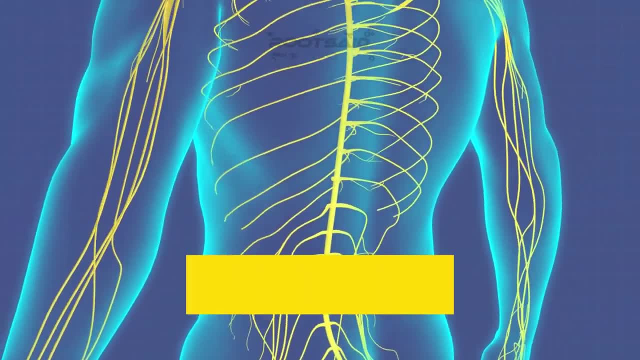 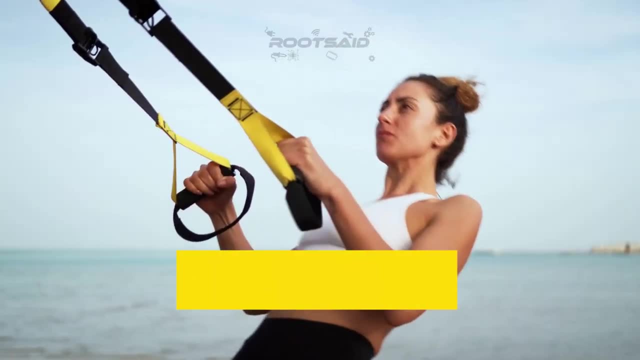 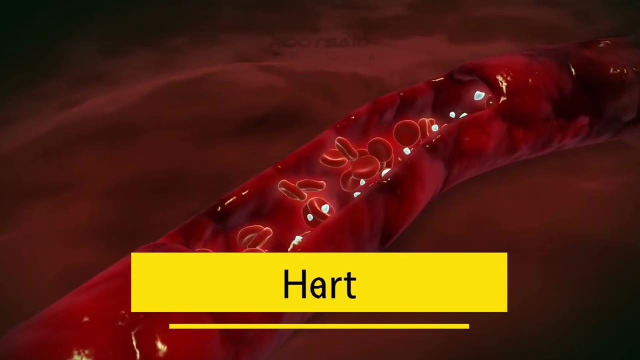 Our neurons transmit these signals from our sense organs to our brain, where we process these external information. Our brain processes the signal, makes a decision and sends the signal to our muscles to move your hands, legs or do whatever you want. We have a heart that circulates blood, supplies oxygen and provides energy for the working of our entire system. 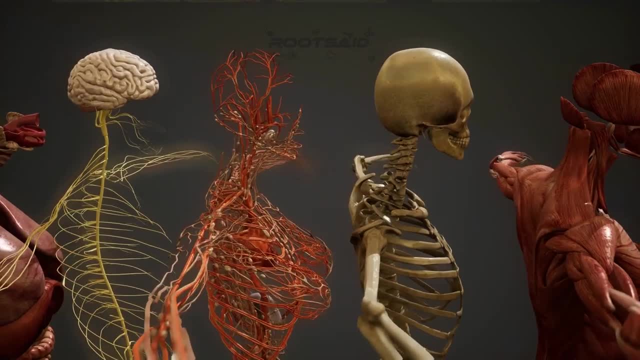 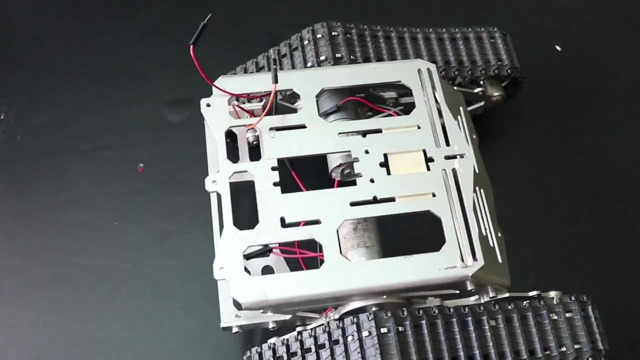 Then we have a body where these sensors, muscles, heart veins and all other parts are neatly assembled. This is the same as in the case of a robot. A robot has a chassis or a robot frame which is similar to our body. 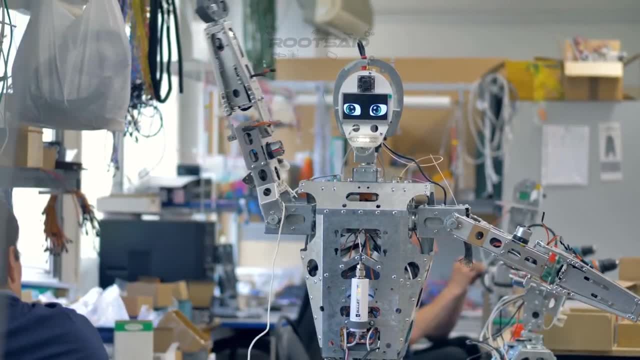 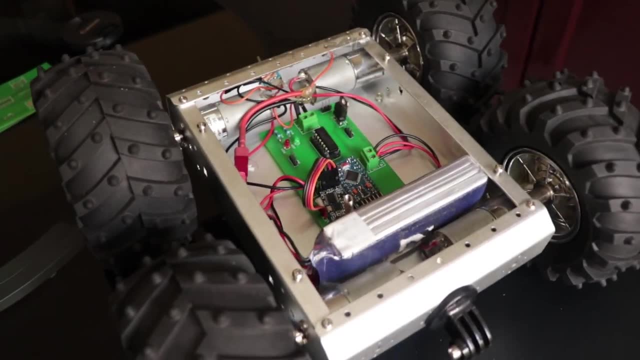 A frame that will support the whole robot, A system which is having enough space and is capable of handling the weight of all. All the sensors, power source and all the cables used in the robot: The sense organs. A robot has sensors. 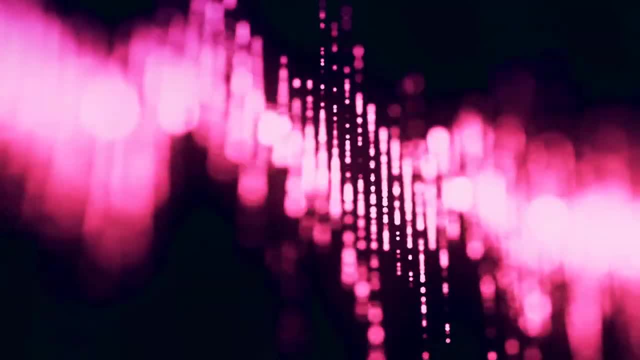 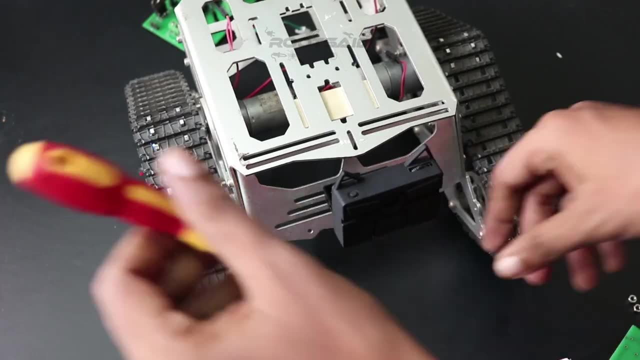 Sensors such as IR sensor, which will sense infrared rays, ultrasonic sensors to sense ultrasonic waves, heat sensors to sense temperature, a pressure sensor to sense pressure or touch, and so much more. Now we have all the data from the sensors, So what to do with this sensor data? 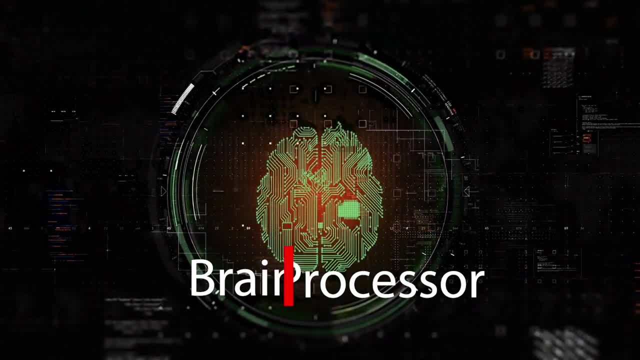 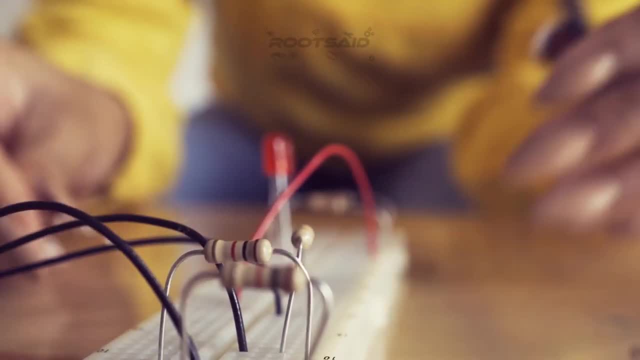 We need to process it. For that we will be having a processing unit. Normally, we will use a logic circuit. This can be a simple circuit consisting of resistors, capacitors, transistors to perform simple logical decisions, or a microcontroller, which is where Arduino comes into play. 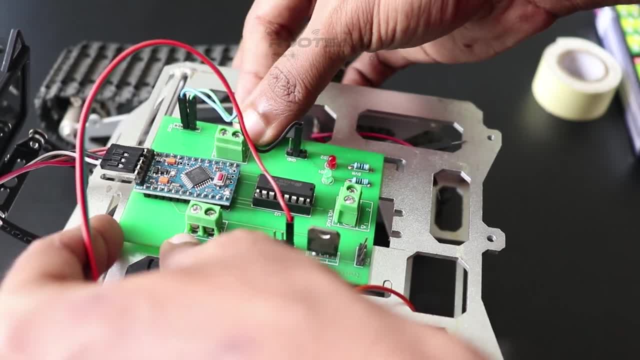 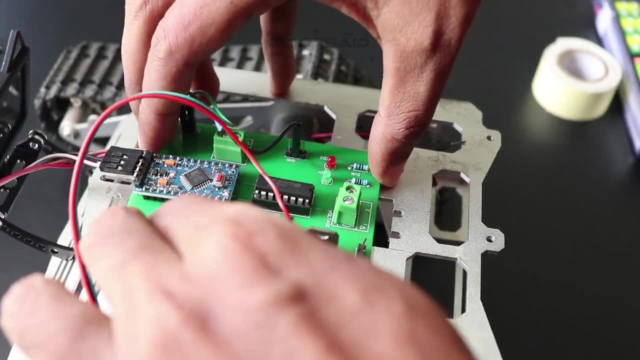 So what exactly is Arduino? I think the best way to explain what Arduino is to start with what you can use it for. Basically, it is a tool for controlling electronics. Well, let me define two general groups of electronic stuff. We have got inputs, and those would be electronic devices. 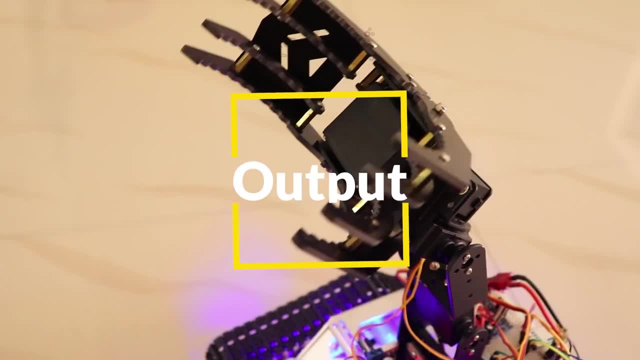 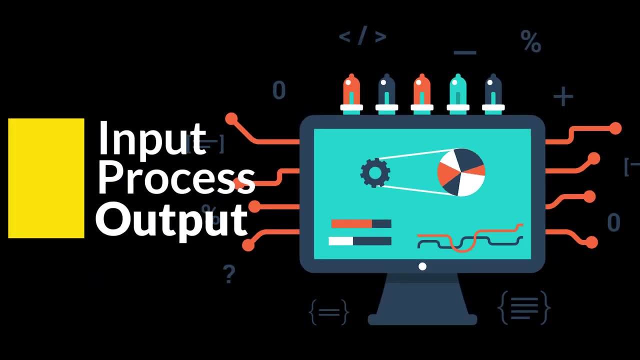 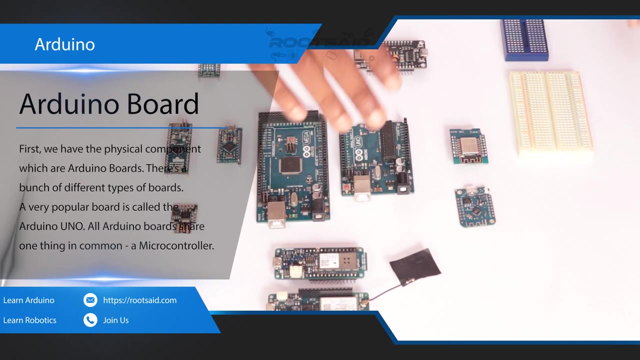 That gather information, like sensors, and we have outputs. those would be electronic devices that do things, like motors, To do something meaningful. we take input from a sensor, process it and do an output. So how do we process it? For that we have the physical component, which contains microcontroller chip called Arduino board. 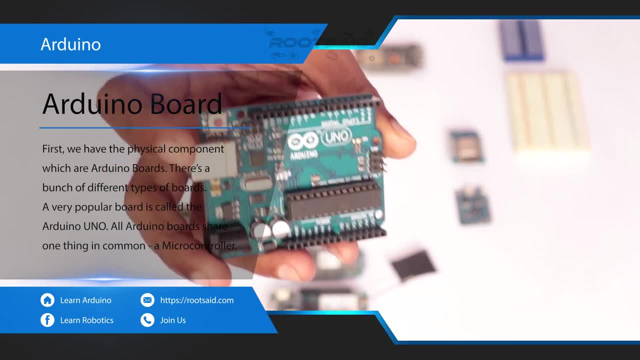 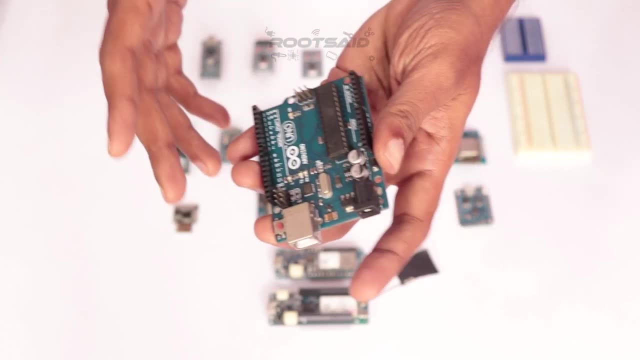 A very popular Arduino board is Arduino Uno. All Arduino boards share one thing in common, and that is they all have a microcontroller on them, And a microcontroller is basically a really small computer which processes the signal and gives output signal to motors and other output devices. 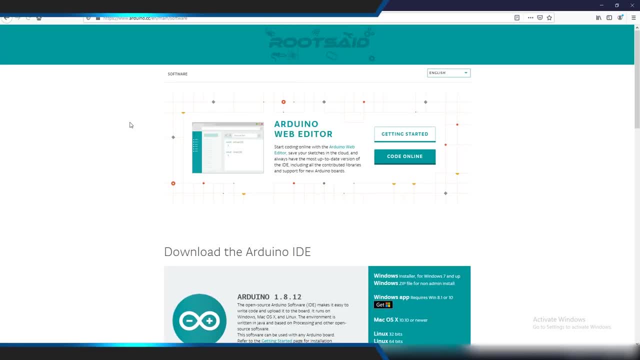 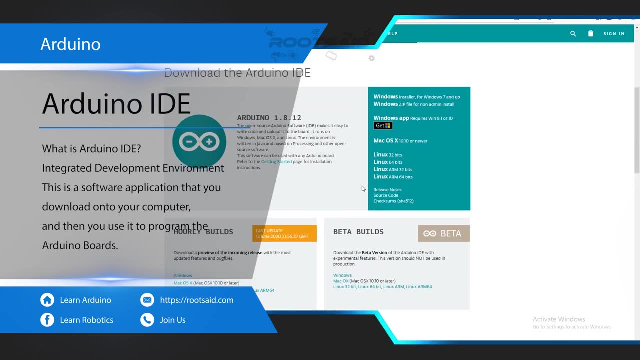 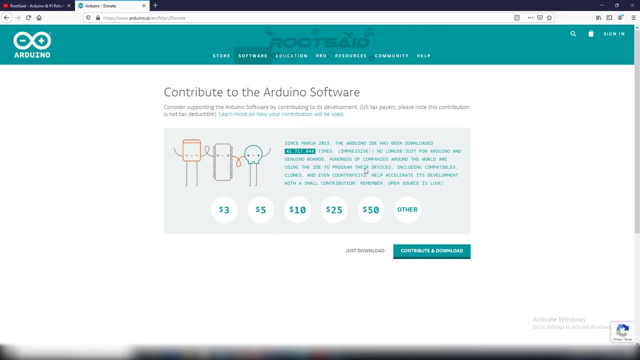 But Arduino is more than just a hardware. it is also a software. There is a thing called Arduino IDE. What is Arduino IDE, you ask? IDE stands for Integrated Development Environment, And this is a software application that you download into your computer and then you use it to program Arduino boards. 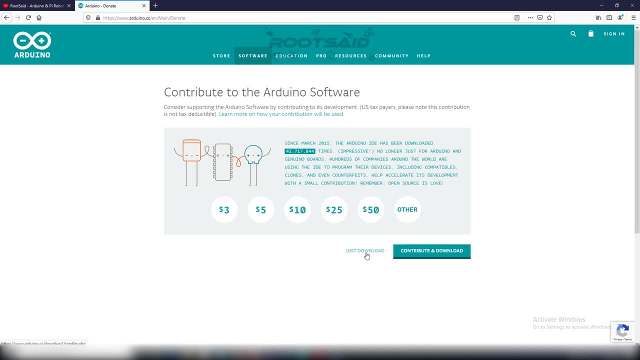 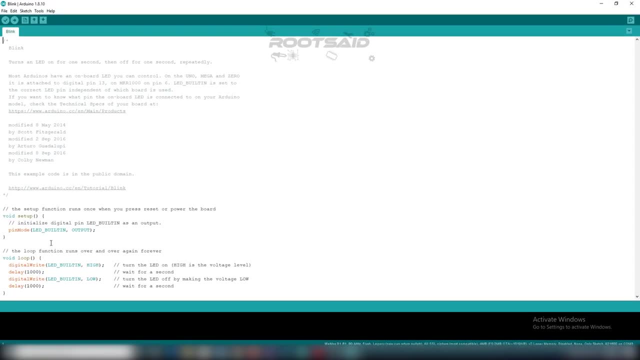 Now it is a completely free software And it is already easy to use. It looks a lot like a text editor. The Arduino IDE is where you write your code that actually gets loaded into your Arduino board itself. The third part of the Arduino is the code. 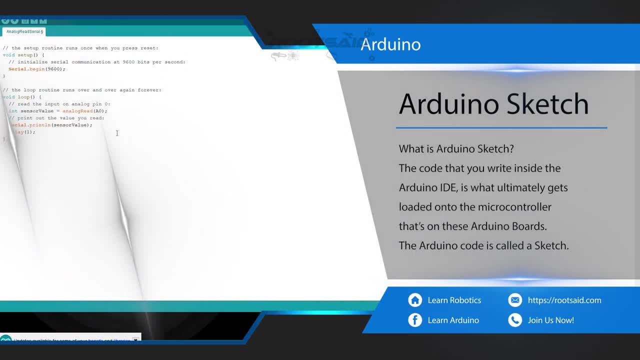 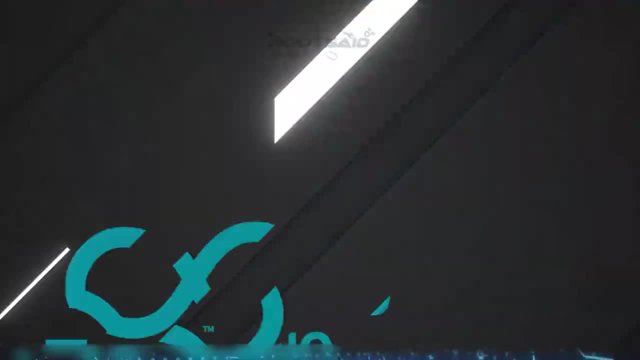 The code that you write inside Arduino IDE is what ultimately gets loaded onto microcontroller. that's on these Arduino boards, And the Arduino code that you write is called a sketch. So what is Arduino? It's three things. There is a physical hardware that uses microcontroller. 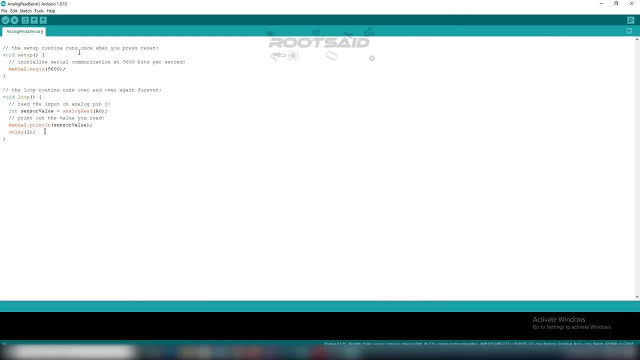 There is the Arduino development engine, There is a development environment called Arduino IDE, And then there is a code itself that's called Arduino sketch, which gets loaded onto the board. Those are the three components that basically make up Arduino. So what makes Arduino best for beginners? 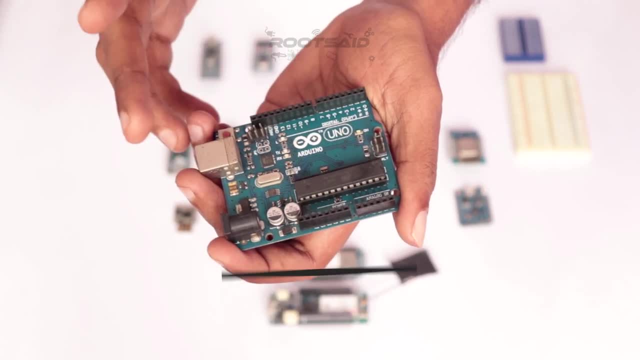 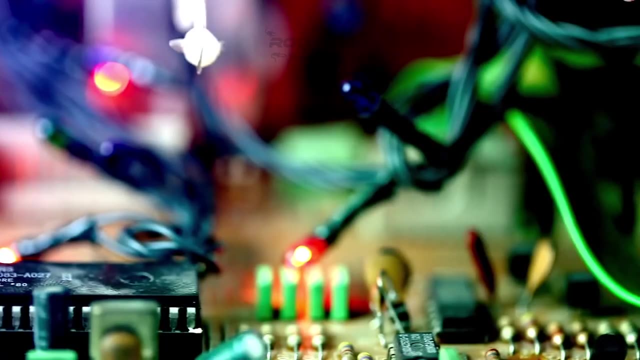 First, the Arduino board itself is designed for ease of use. You can connect it to your computer with a simple USB cable and not with special cable that it would normally take to connect a microcontroller. Connecting electronic components to the microcontroller is also very easy with an Arduino board. 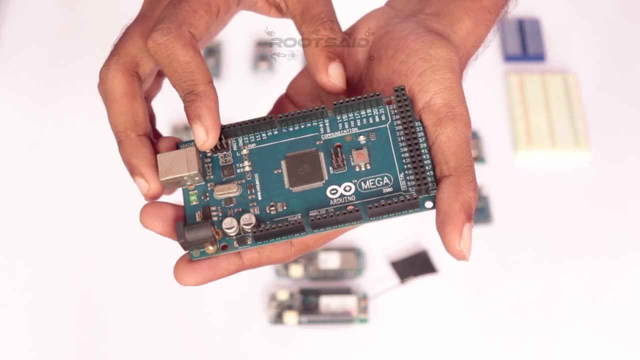 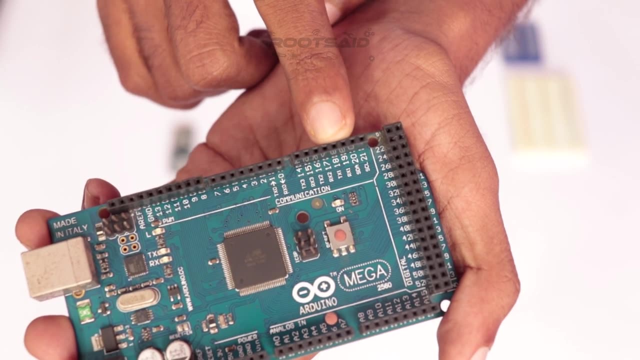 Because they have these plastic holes around the perimeter of the board. They are called headers- And to connect an electronic component to the microcontroller you just stick the component inside the holes. It's literally that easy. This board also has a built-in external power jack. 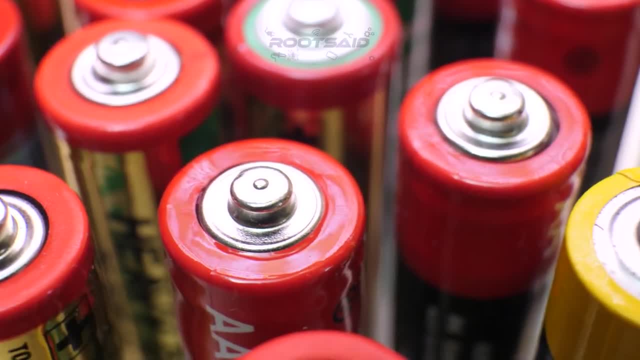 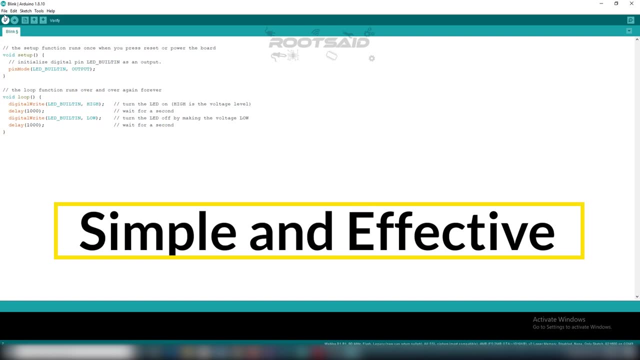 So when it's not hooked up to the computer, it can still be powered by a battery pack. The Arduino IDE is also designed for ease of use. There is a lot of integrated development environment out there, but Arduino IDE is built with simplicity in mind. 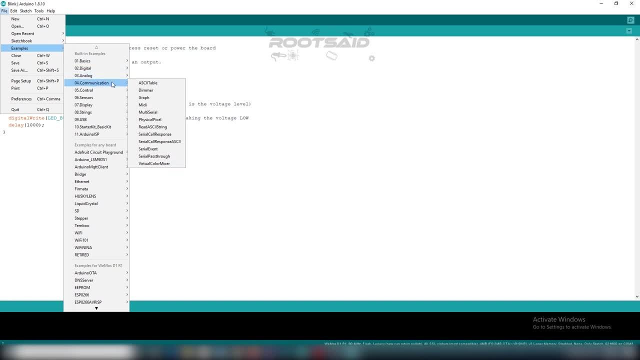 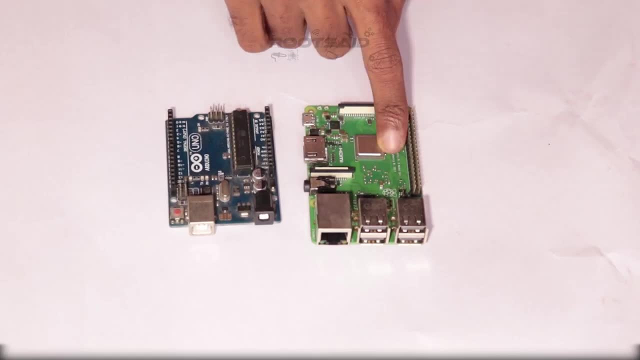 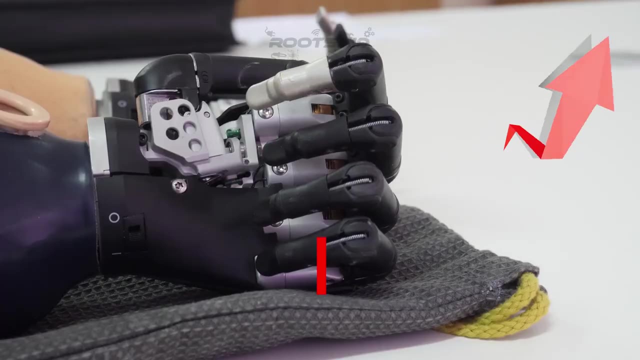 It's really just a basic window where you type your code and to upload the code you have written, you simply press a button and that's it. Arduino and Raspberry Pi are the most commonly used controllers in the field of DIY robotics. Check out this playlist if you want to learn more about Arduino motors and other moving parts as muscles. 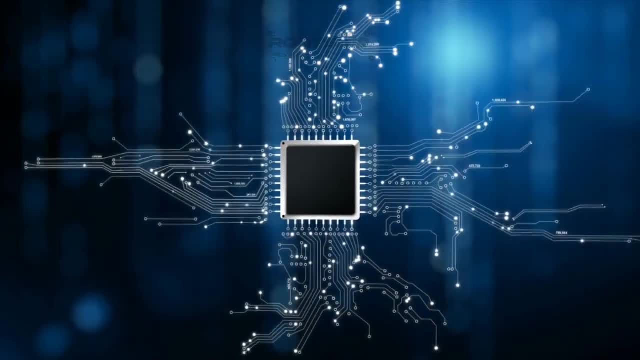 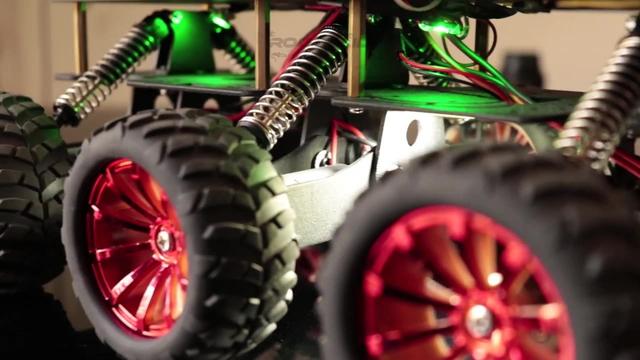 Once the signals are being processed by the microcontroller, the result or reaction will be sent to the actuators. Actuators can be any electromechanical device, such as motors that will move the robot, or servo motors that will lift the hand, or anything that performs a physical action. 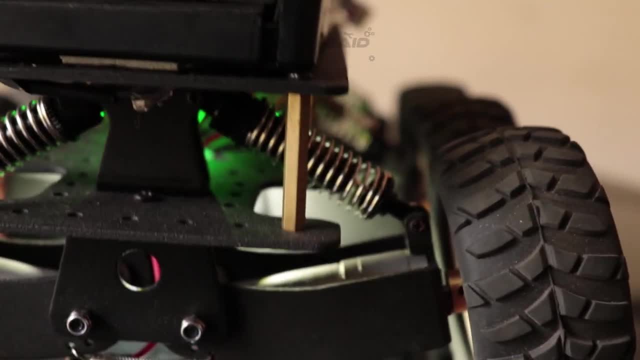 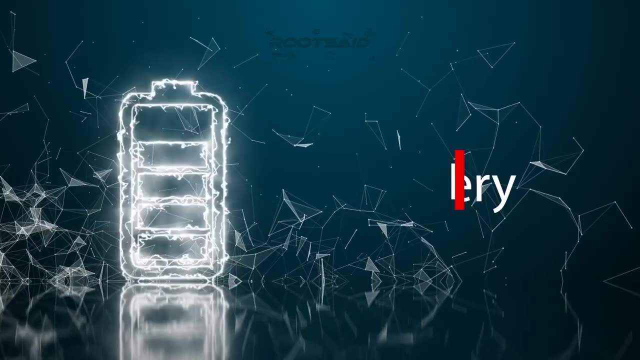 Motors are one of the most commonly used actuators used in robots. This is also the best actuator from which kids can start learning robotics and programming. The battery as the heart. Now we almost have everything we need now. All we need is a power source. 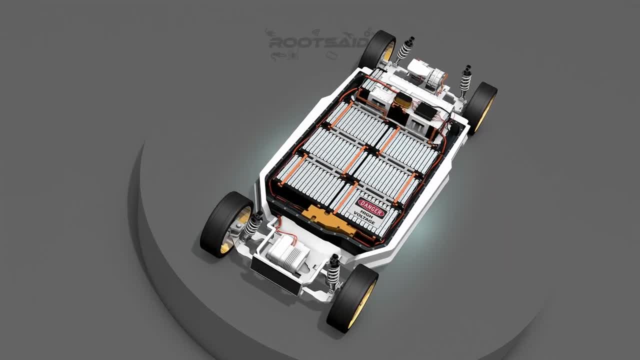 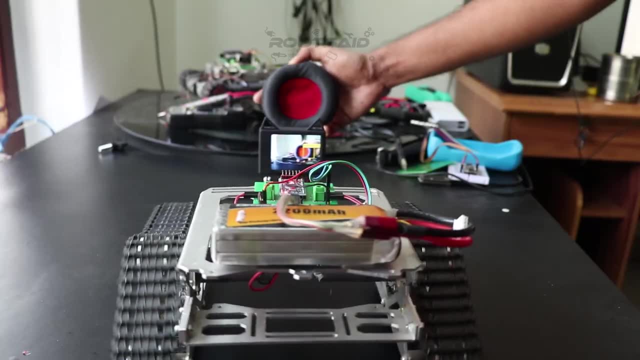 A power source that can provide enough energy to power up all the sensors, motors and microcontroller. For that we will use a current source such as a battery or a power adapter. Basically, this is what a robot is. Everything is good with an example, right? 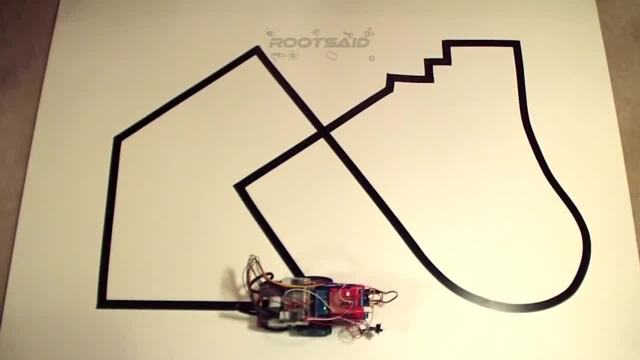 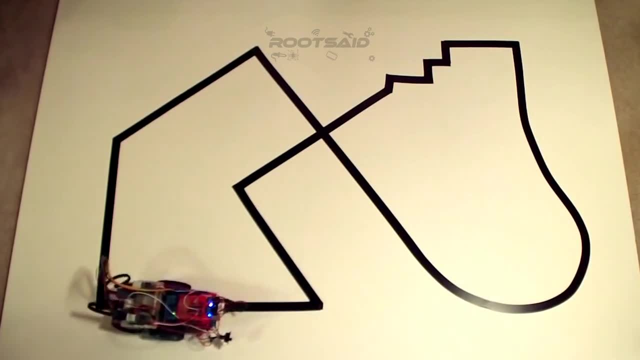 So let's see one DIY robot in action. Consider this line following robot using Arduino. This robot uses IR sensor to detect the track and use motors to move around depending upon the color of the track. Here, the IR sensor is the sensor that senses the environment and gathers input. 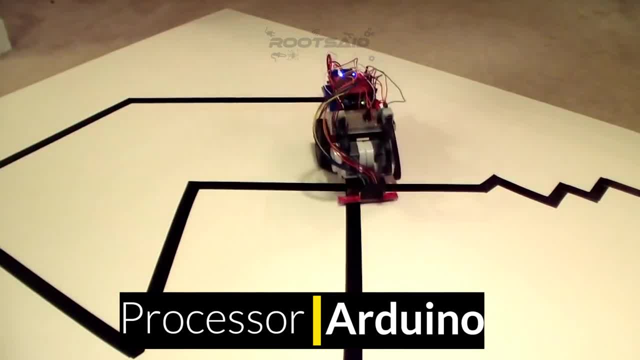 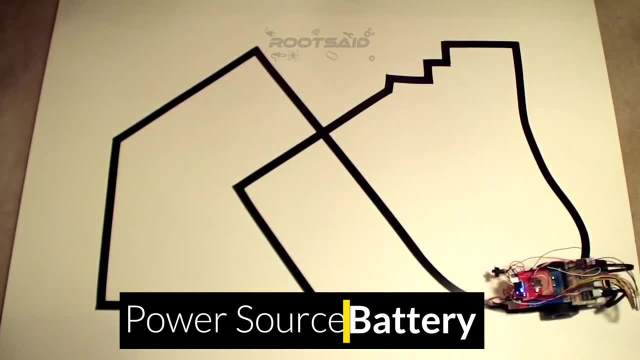 Arduino is the brain that processes the input signal and generates signal to control output devices. Motors are like the muscles that do the desired action. Battery is the heart that powers the whole circuit. Robot chassis is the body where we assemble all the body parts. 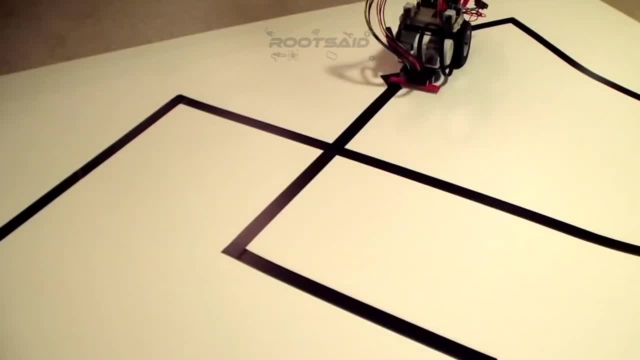 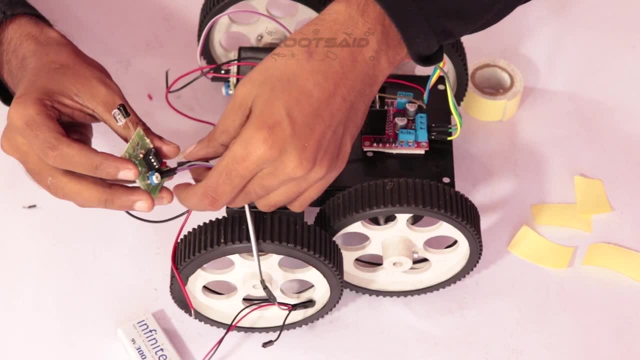 Using all these parts, the robot senses the path, takes a decision by its own and reacts to its environment by moving only through the black path. The most basic autonomous robot you can build in your home is a line follower. You can make a line follower with or without a microcontroller.